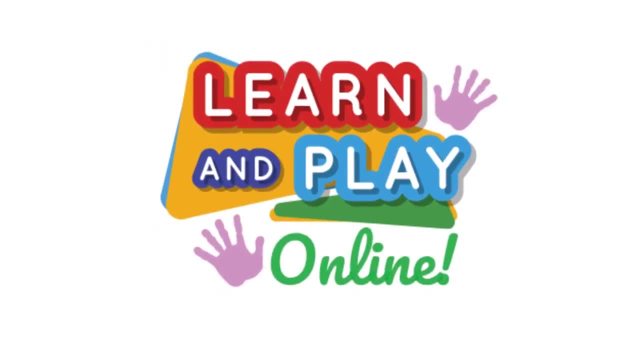 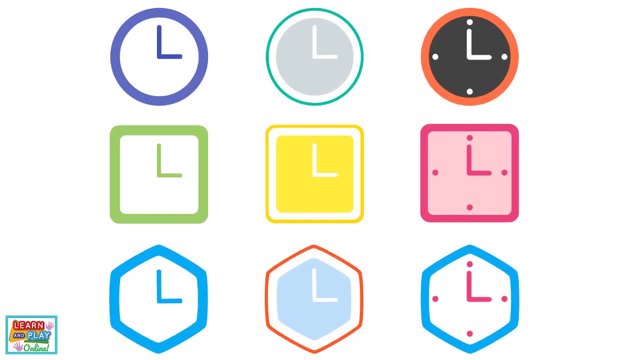 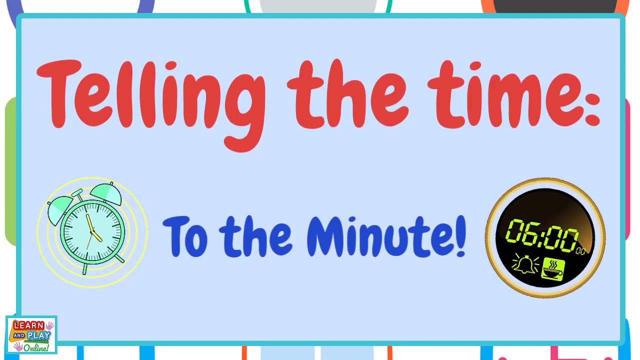 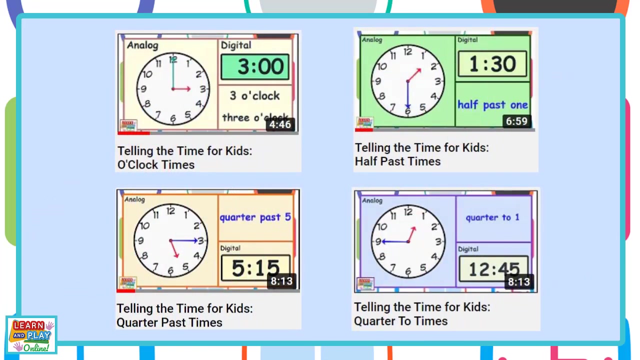 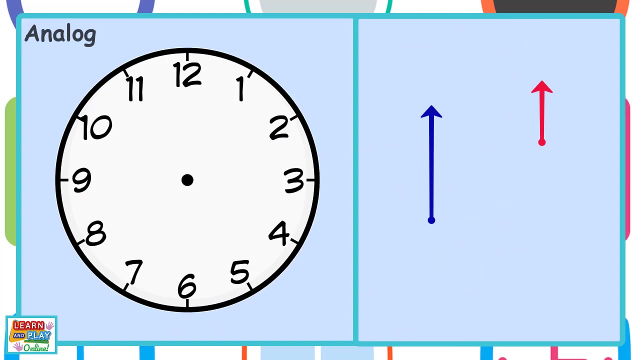 Please check out our other time videos if you haven't already seen them. Click on the links in the description box. Here are the two hands for our clock face. Remember that the long hand is called the minute hand and the shorter hand is called the hour hand. 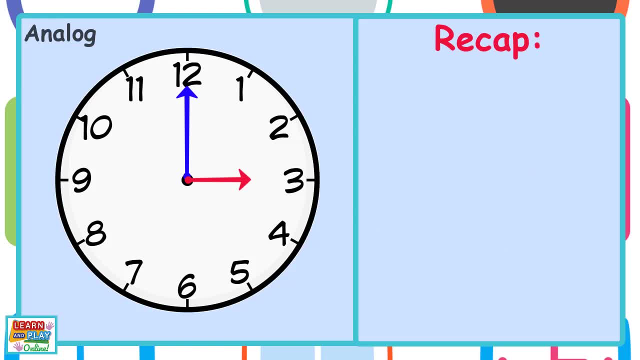 Before we continue, let's recap on what we already know. There are 60 minutes in one hour. There are 30 minutes in half an hour. So that means there are 15 minutes in a quarter of an hour. When the minute hand is pointing at the 12, we say it is something o'clock. 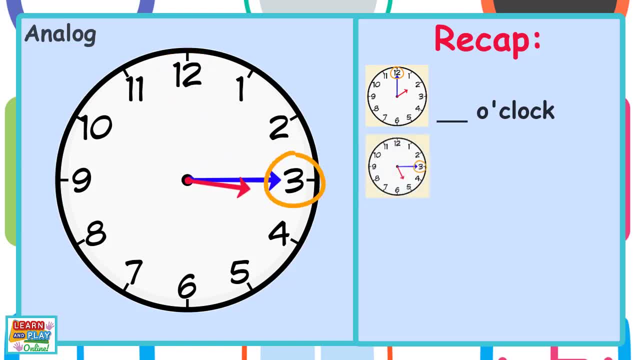 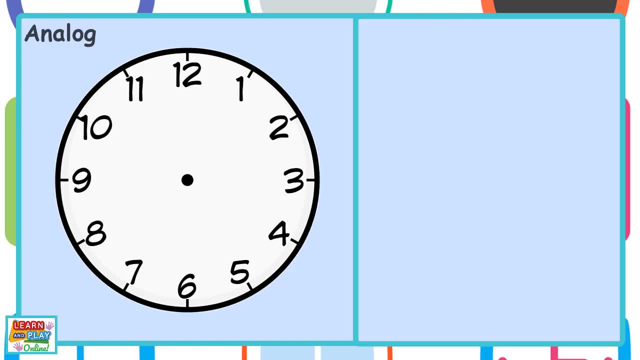 In this video, we are going to learn how to read time on an analogue clock to the minute. To do this, we will need to use a different clock face. You will notice that this new clock face has these little lines in between the numbers. 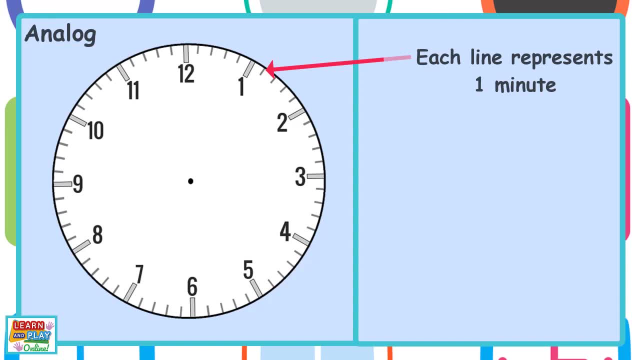 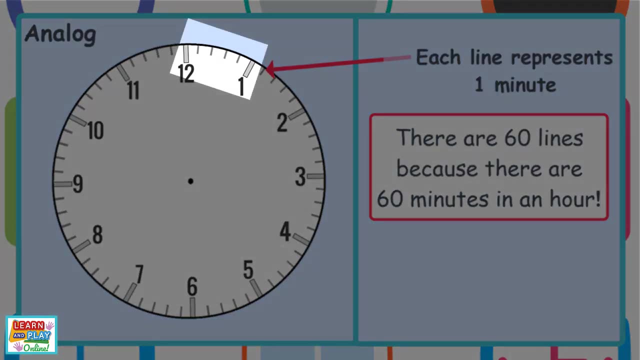 Each line on the clock face, including the ones with the numbers, represents one minute. There are 60 lines on the clock face because there are 60 minutes in an hour. Notice that there are four little lines in between each number on the clock face. 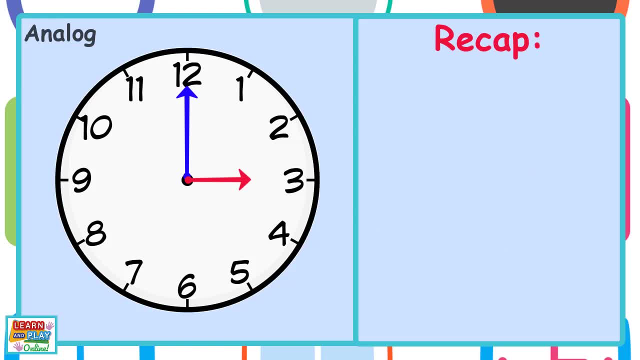 Before we continue, let's recap on what we already know. There are 60 minutes in one hour. There are 30 minutes in half an hour. So that means there are 15 minutes in a quarter of an hour. When the minute hand is pointing at the 12, we say it is something o'clock. 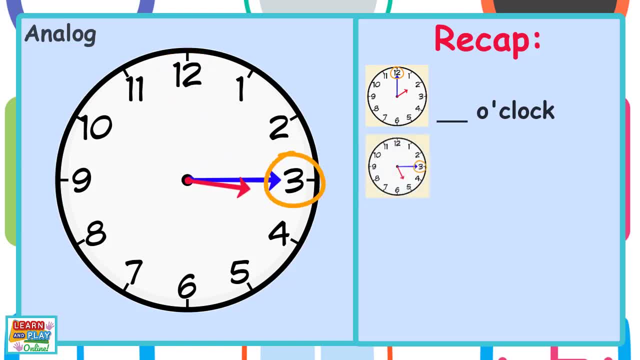 When the minute hand is pointing at the 3, we say it is quarter past something. When the minute hand is pointing at the number 6, we say it is half past something. And lastly, when the minute hand is pointing at the number 9, we say it is quarter to something. 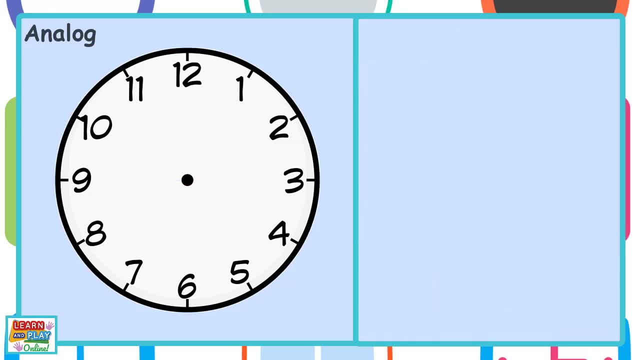 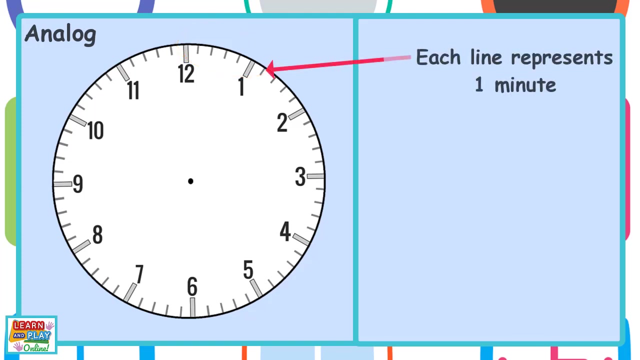 In this video. In this video. In this video, we are going to learn how to read time on an analog clock to the minute. to do this, we will need to use a different clock face. you will notice that this new clock face has these little lines in between the numbers. each line on the clock face, including the ones with the numbers. 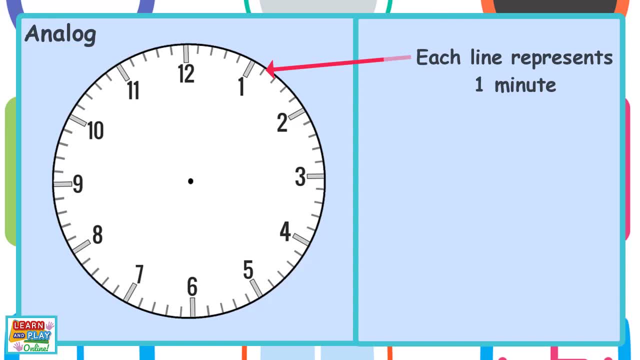 represents one minute. there are 60 lines on the clock face because there are 60 minutes in an hour. notice that there are four little lines in between each number on the clock face. this means that we can count by increments of five minutes each time we reach one of the numbers on the clock face. 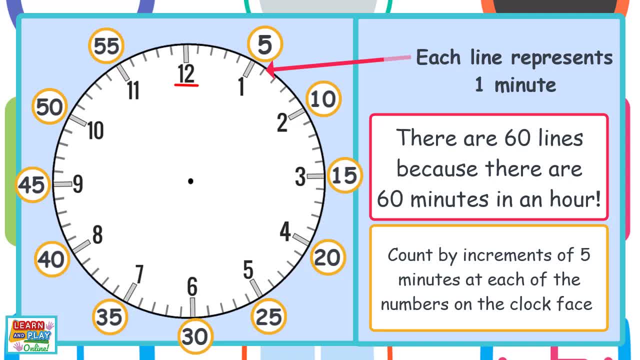 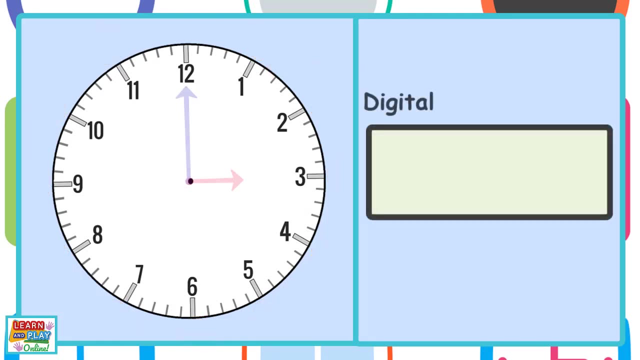 keep in mind that when the minute hand reaches the 12, the minutes will start back at zero. as it is the beginning of a new hour, let's start reading time to the minute so you have a better understanding of this. the time on the analog clock is currently three o'clock. now watch the minute hand closely. 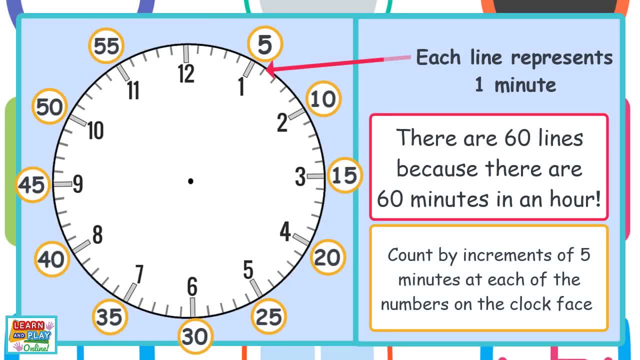 This means that we can count by increments of 5 minutes each time we reach one of the numbers on the clock face. Keep in mind that when the minute hand reaches the 12, the minutes will start back at zero, as it is the beginning of a new hour. 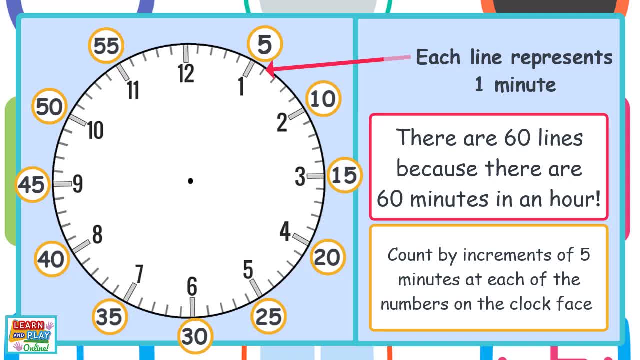 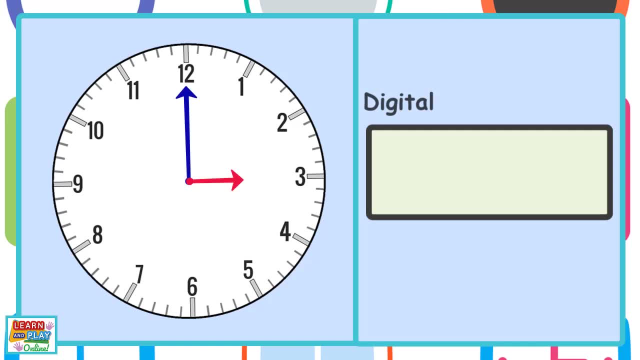 Let's start reading time to the minute so you have a better understanding of this. The time on the analogue clock is currently 3 o'clock. Now watch the minute hand closely as it moves to the next minute. That means the time is now 3.01.. 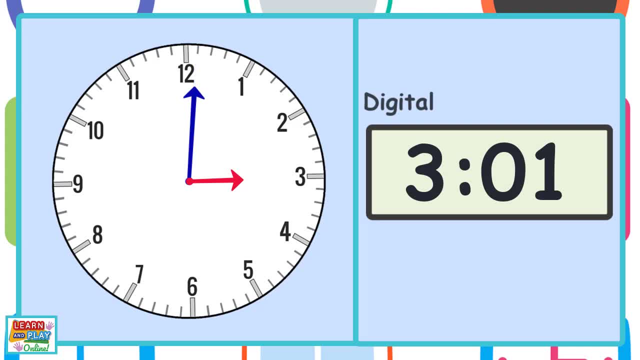 Let's watch the minute hand move to the next minute. again Now the time is 3.02.. Next is 3.03,, then 3.04, and then 3.05.. You can see and understand now that when the minute hand is pointing at the line at the number 1, that shows that 5 minutes has passed the hour. That means the time is now 3 o'clock. You can see and understand now that when the minute hand is pointing at the line at the number 1, that shows that 5 minutes has passed the hour. 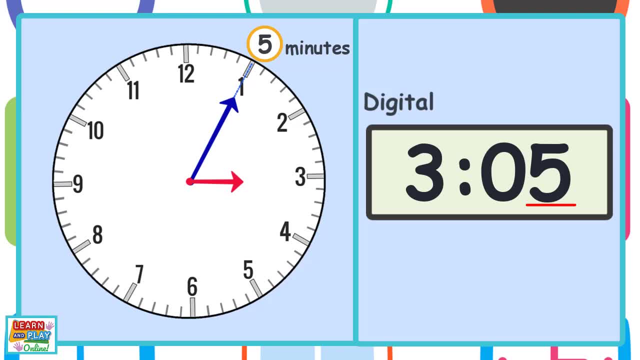 You can see and understand now that when the minute hand is pointing at the line, at the number 1, that shows that 5 minutes has passed the hour. Using this strategy of counting by increments of 5 minutes will be a much faster way to. 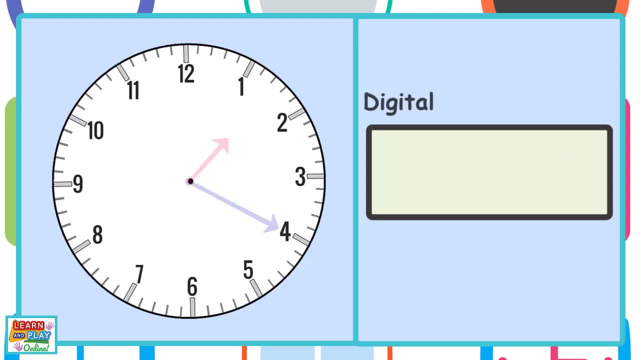 read time. Let's give this a go. First of all, we need to look at the hour hand. It has gone past the number 1, so it is 1 something. Now let's look at the minute hand. It is pointing at the line, at the number 4, so let's count by 5s around the clock face. 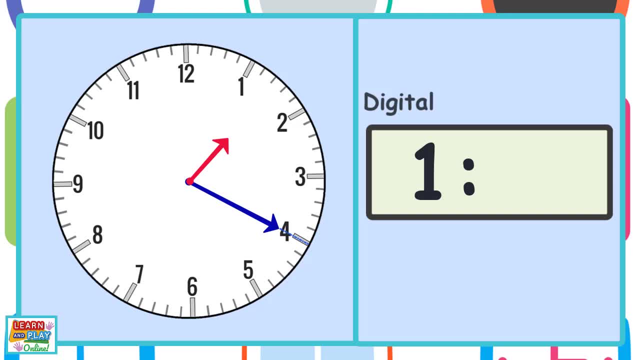 until we reach the number 4 to find out how many minutes have passed the hour. 5,, 10,, 15,, 20,. oh, so that means 20 minutes has passed the hour, so the time is 1.20.. 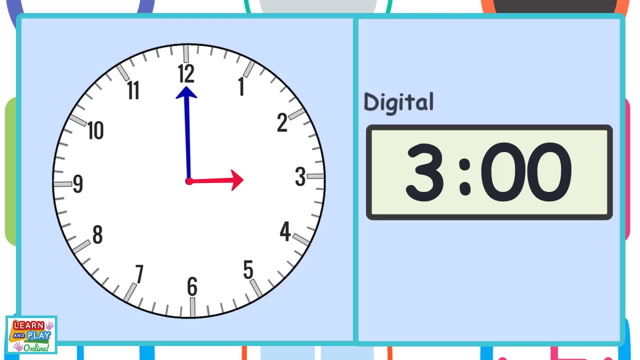 as it moves to the next minute. that means the time is now 301. let's watch the minute hand move to the next minute again. now the time is 302, next is 303, then 304 and then 305. you can see and understand now that when the minute hand is pointing at the line, at the number, 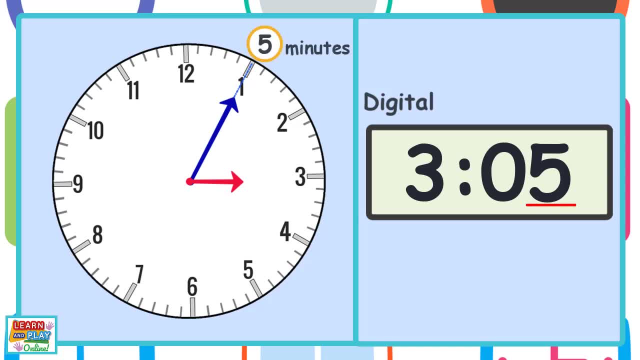 one that shows that five minutes has passed the hour. using this strategy of counting by increments of five minutes will be a much faster way to read time. let's give this a go. first of all, we need to look at the hour hand. it has gone past the number one, so it is one something. 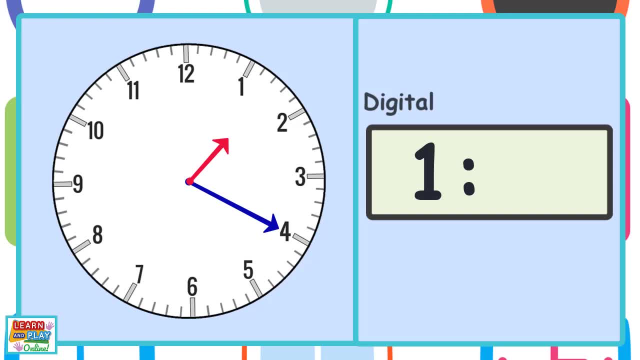 now let's look at the minute hand. it is pointing at the line, at the number four. so let's count by fives around the clock face until we reach the number four to find out how many minutes have passed the hour. five, ten, 15, 20. 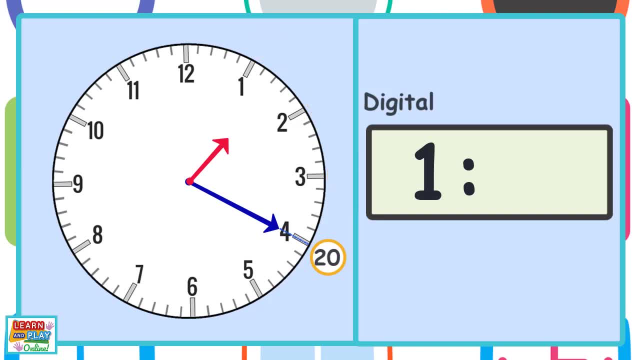 5, 10, 15, 20. oh so that means 20 minutes has passed the hour, so the time is 120.. let's try the next one. remember we always need to look at the hour hand first. the hour hand is past the number 10, so it must be 10 something. 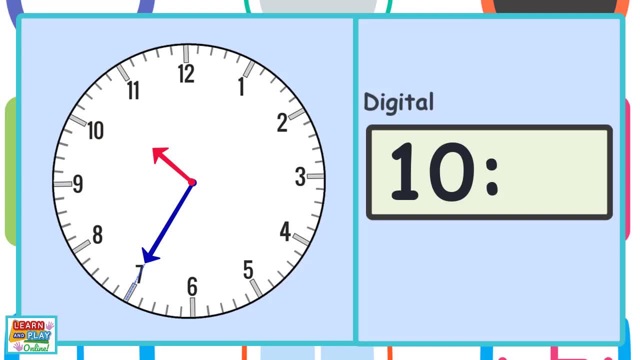 the minute hand is pointing to the line at the number, So let's count by 5's around the clock face to see how many minutes has passed the hour: 5, 10, 15, 20, 25, 30, 35. So that means the time is 10.35.. 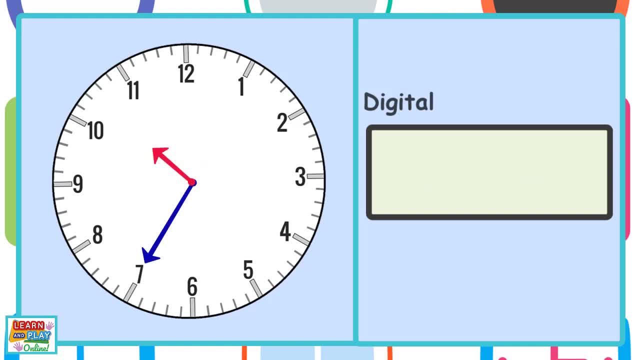 Let's try the next one: 1.20.. 1.20.. The time has passed the hour, since the hour hand is pointing at the line at the number 1.. If you count by this experiment, you are given 10 minutes to read, so remember, we will count. by 5s around the clock face until we reach the line at the number 7.. Oh, and, in the case of the hour hand, we can change it to 5s around the clock face, just to check the time given along the clock face. 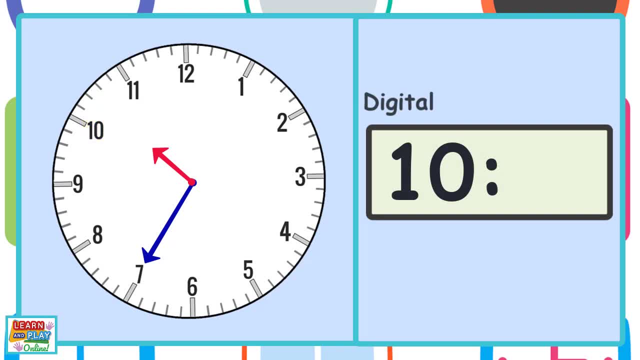 It has passed the number 10, so the time is 1.10.. So it must be 10 something. The minute hand is pointing to the line at the number 7, so let's count by 5s around the clock face to see how many minutes has passed the hour. 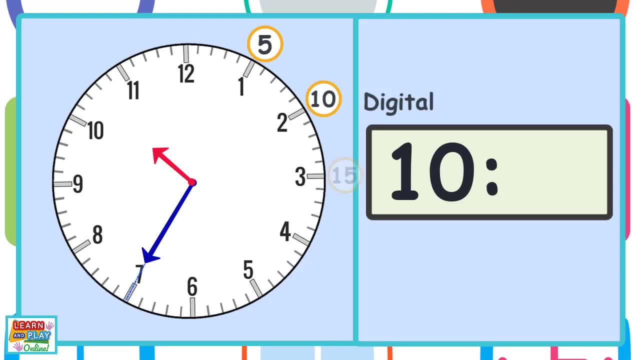 5, 10,, 15,, 20, 25.. Ok, this is symbol. so where is this number? 1.20.. thirty thirty five, so that means the time is ten thirty five. looking at the hour hand, it is past the number four, so it is for something now. 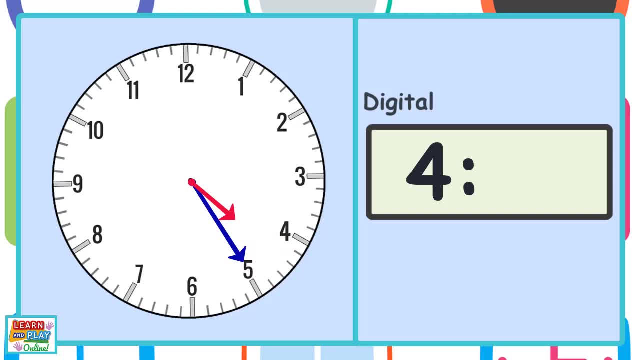 I'm going to count by fives until I reach the line at the number five to find out how many minutes has passed the hour five, ten fifteen twenty twenty five, so the time is 425. in this time we can see that the hour hand is still in the 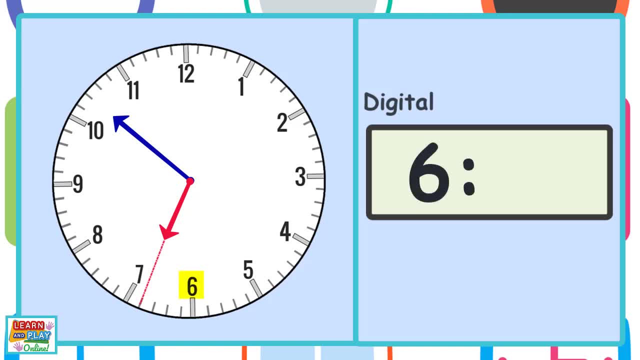 sixth hour, so it is six something, as it has not yet reached the number seven. you can see that the minute hand is pointing to a little line that is not at a number on the clock face. this means we will first count by fives until we get to the number ten on. 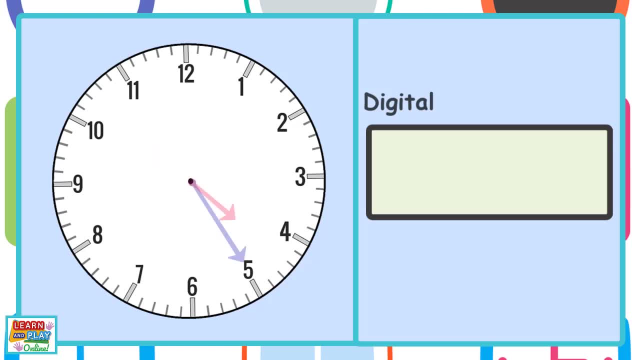 Looking at the hour hand, it is past the number 4.. So it is 4 something. Now I'm going to count by 5's until I reach the line at the number 5 to find out how many minutes has passed the hour. 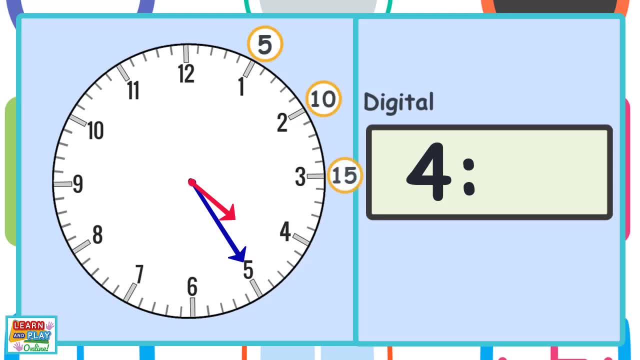 5, 10, 15, 20, 25, So the time is 4.25.. In this time we can see that the hour hand is still in the 6th hour, So it is 6 something, as it has not yet reached the number 7.. 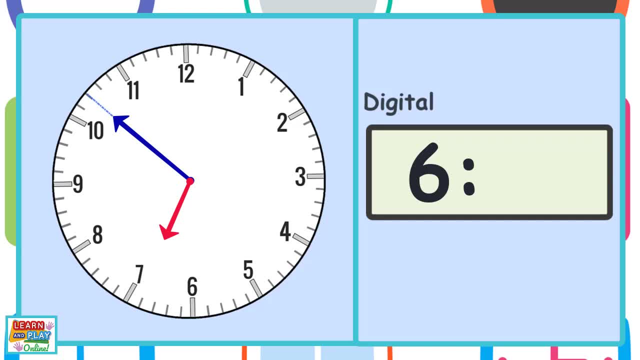 You can see that the minute hand is pointing to a little line that is not at a number on the clock face. This means we will first count by 5's and then we will count by 5's Until we get to the number 10 on the clock face and then count by 1's. 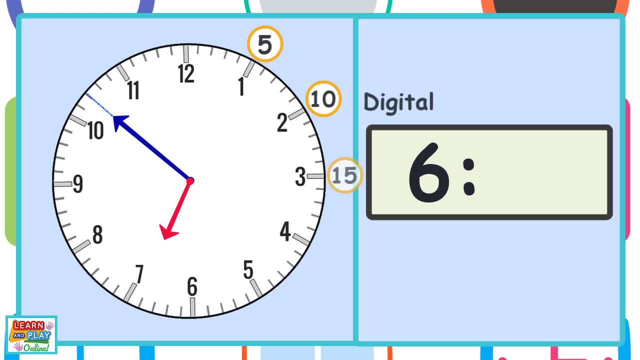 5, 10, 15, 20, 25, 30, 35, 40, 45, 50, 51, 52. So that means that the time is 10.35.. The time is 6.52.. Let's try one last time. 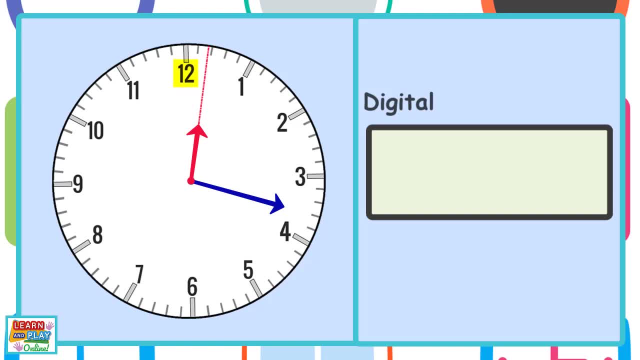 The hour hand is past the 12.. So it is 12 something. Now let's find out how many minutes has passed the hour. 5, 10, 15, 16, 17, 18. So the time is 12.18.. So the time is 12.18.. 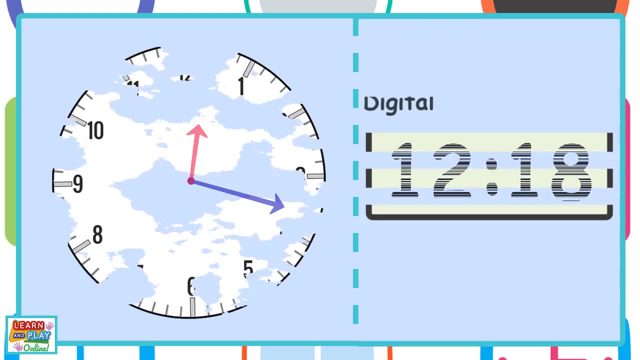 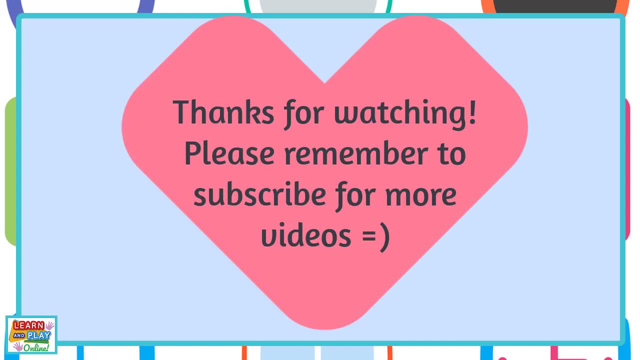 So the time is 12.18.. Thanks for watching. Please remember to subscribe for more videos.